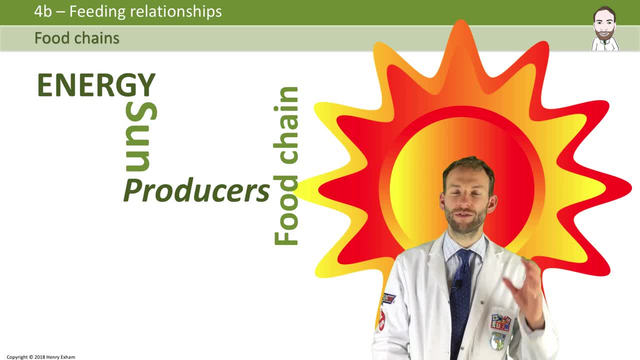 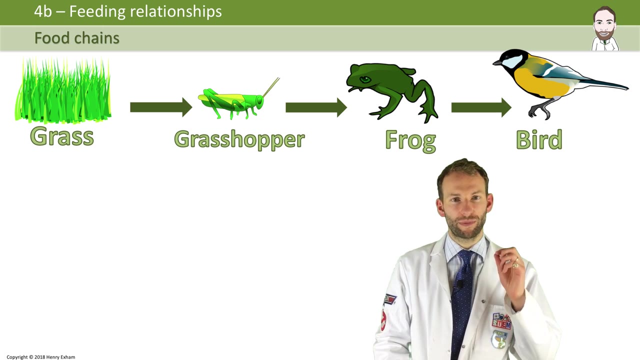 basically. So we don't put the sun in any food chain. We don't show the sun there because it's not part of the food chain. It's not food, but it's important to realize that the sun is the source of the energy. Here is a typical food chain. We've got grass, grasshopper, frog and bird, Now plants. 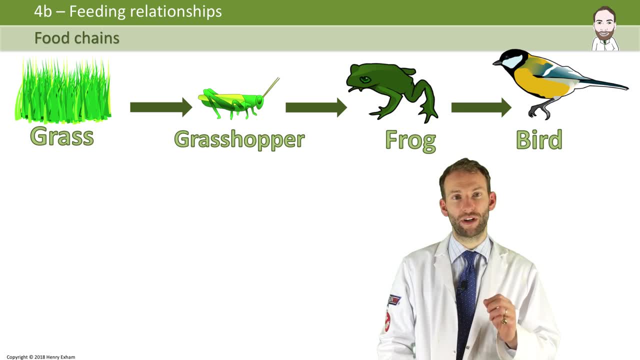 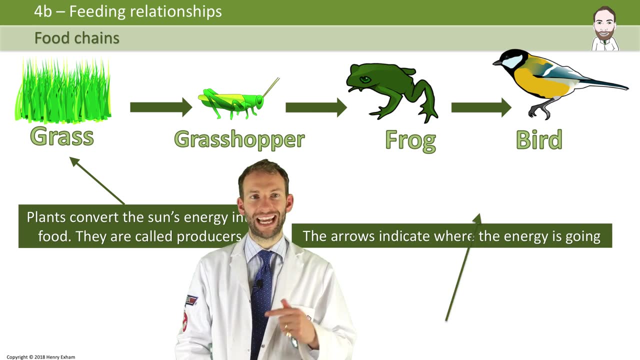 convert the sun's energy into food, as we've just said. Therefore, we call the plant the producer, because it's producing the energy. The arrow indicates where the energy is going. So that's what the arrows show in a food chain. It shows the energy flow. Each stage in a food chain is called. 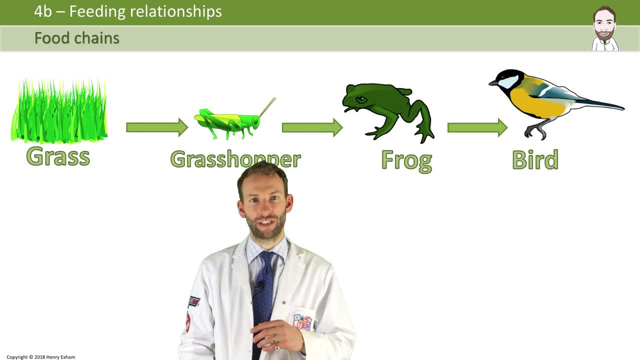 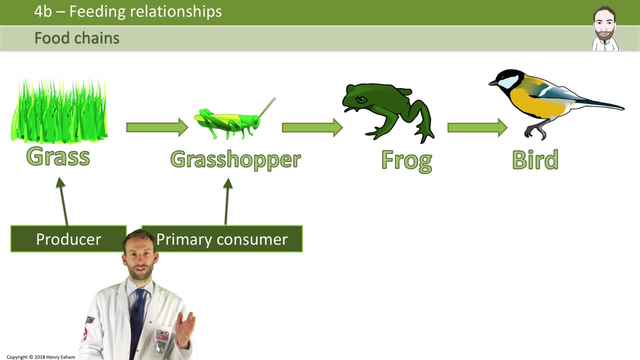 a trophic level. So there are four trophic levels in this food chain and each trophic level has a particular name. We talked about the producer, Then you've got the primary consumer, because the first consumer consumes the grass. We've got the secondary consumer and then you have the tertiary. 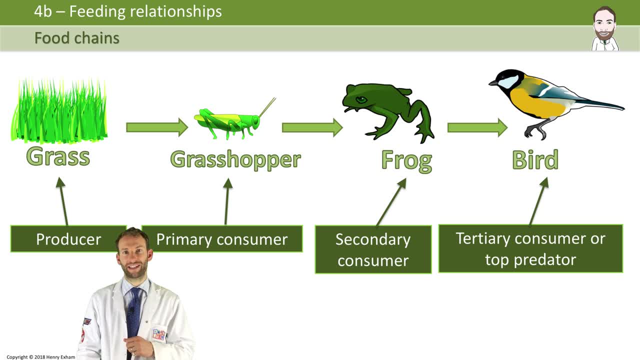 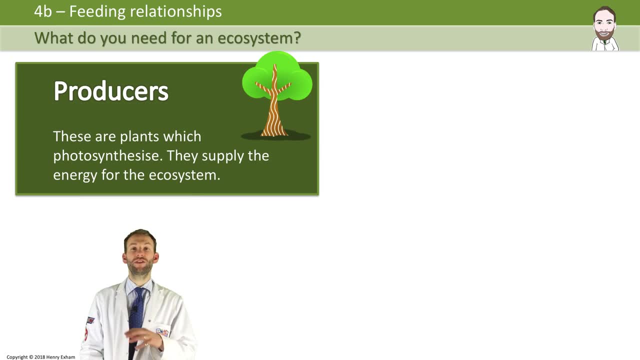 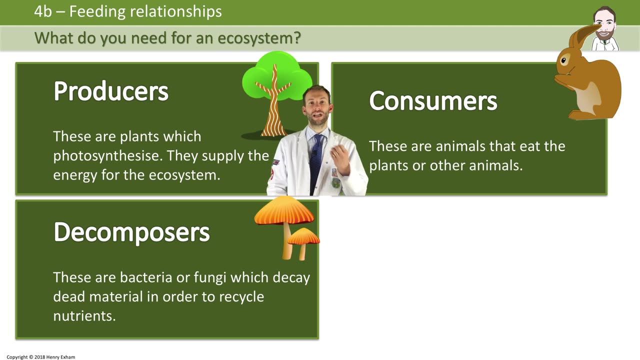 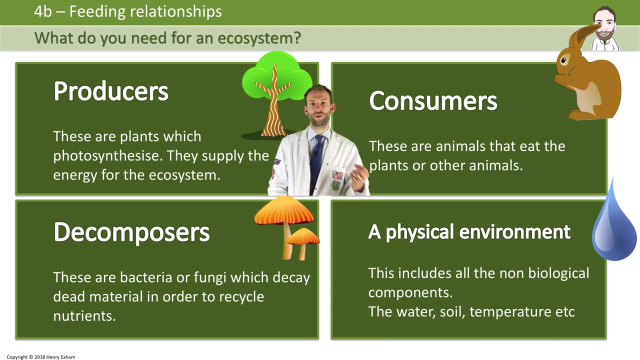 consumer because it's the last thing in the food chain. We call it the top predator. So in order to explain the top predator, we collect corn, corn and phabout the icing, Then we collect all the other nuts from the food chain and we are doing the. work together with the secondary consumer of the food chain. Next, we have a system of food chain. We call it the food chain, We call it a non-biological centric system. Either the physical environment or the Первostrum, It's the organic system where you will have 하나 place where you'll have humanity. 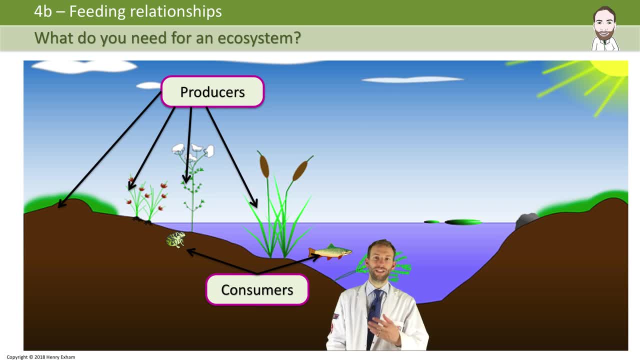 we've got the producers, we've got the consumers, but we've also- and we've got the decomposers in there as well, probably in the soil and some living in the water. but we've also got our abiotic factors. 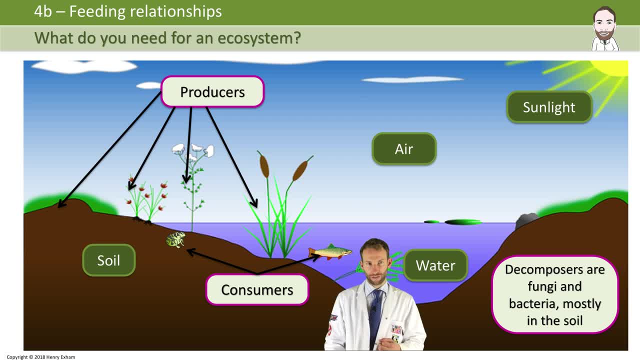 the air, the water, the soil, the sunlight. So all these things work together to form an ecosystem, and an ecosystem is a combination of the living organisms and the physical environment. Now, a herbivore is an animal that just eats a plant. 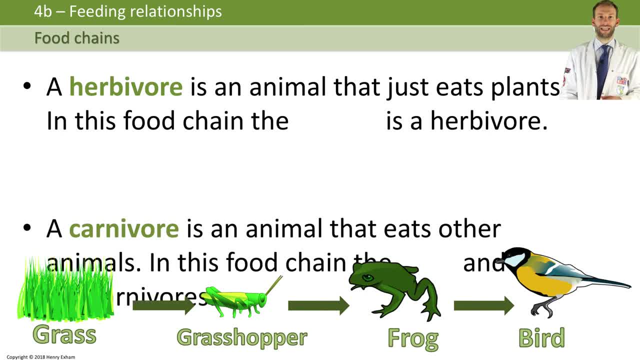 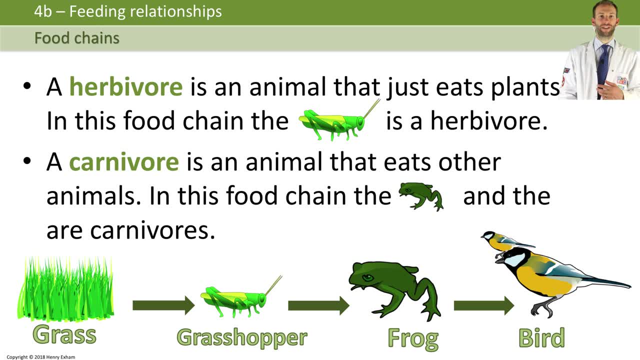 In this food chain. the grasshopper is the herbivore. A carnivore is an animal that eats other animals, So in this case it would be the frog and the bird would be carnivores. If you're an omnivore, you eat both plants and animals.